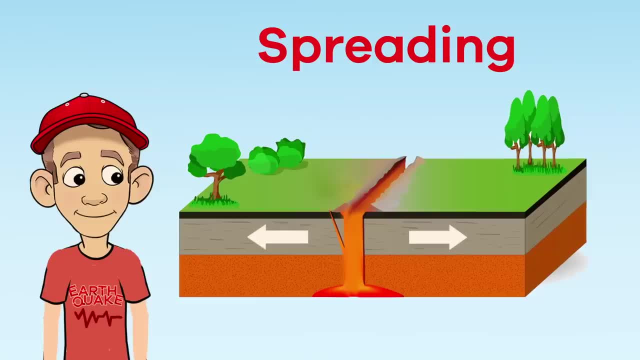 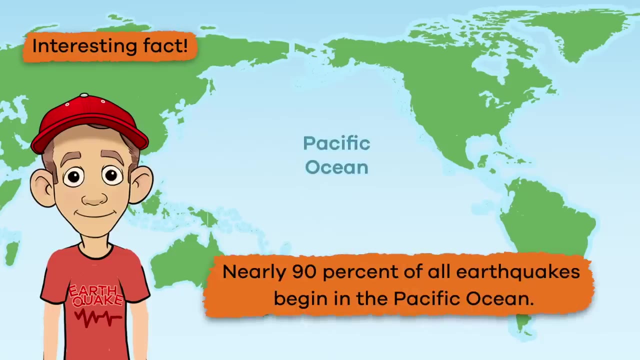 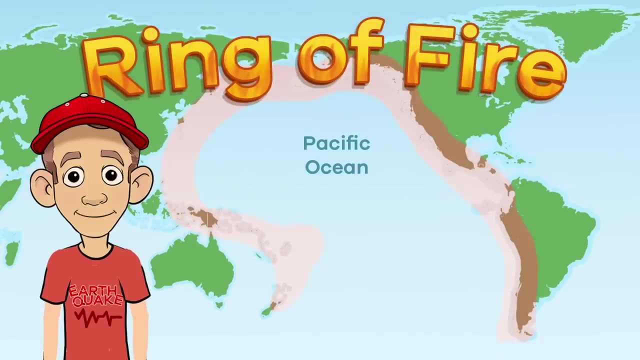 spreading happens when plates move apart from each other. When they do, melted rock between the plates rises and cools, forming new crust. Here's an interesting fact: Nearly 90% of all earthquakes begin in the Pacific Ocean, in an area called the Ring of Fire. It's called the Ring of Fire because, along with earthquakes, 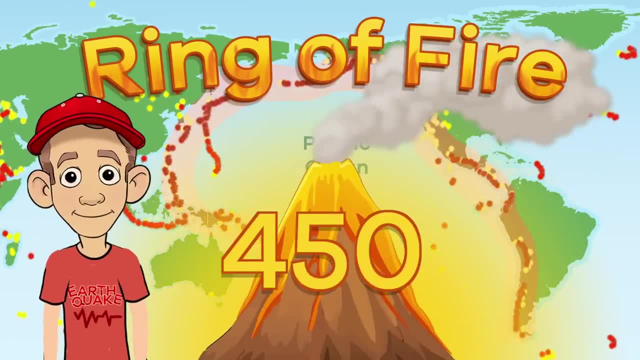 it's filled with many active volcanoes- More than 450!. Earthquakes can be powerful enough to change the course of the Earth's course of movement. Earthquakes can be powerful enough to change the course of the Earth's course of movement. 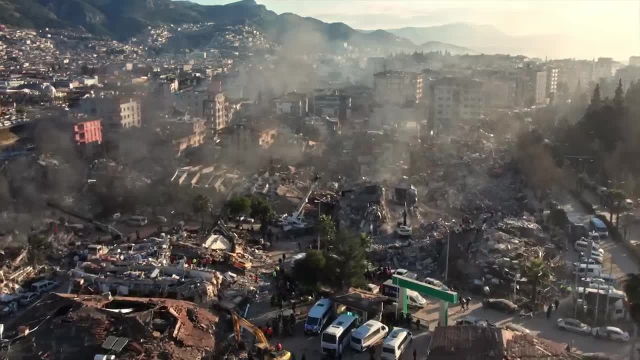 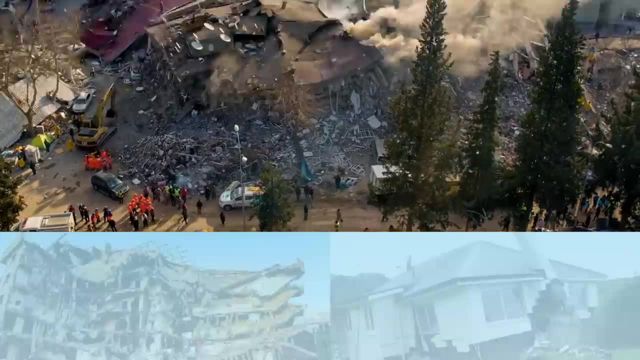 Earthquakes can be powerful enough to change the course of the Earth's course of movement. Earthquakes can change the surface of the Earth and can do a lot of damage, And sometimes earthquakes can even cause other natural disasters like avalanches, landslides and tsunamis. 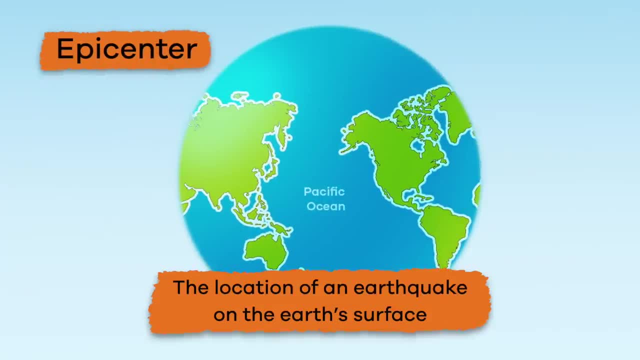 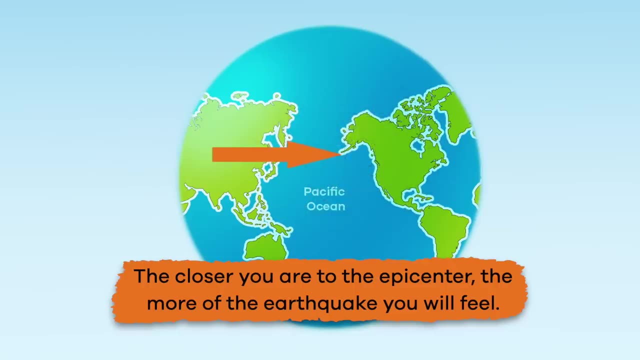 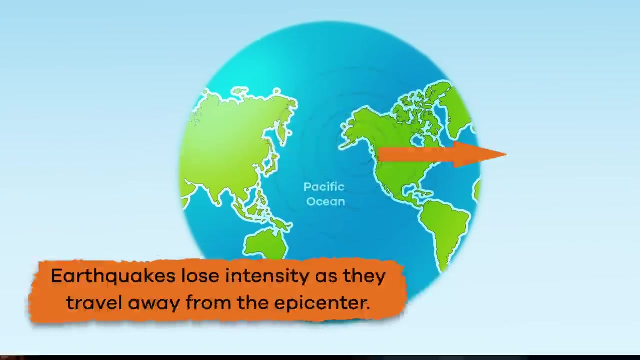 Pretty wild, right. The epicenter is the location of an earthquake on the Earth's surface. The closer you are to the epicenter, the more of the earthquake you will feel. Earthquakes lose intensity as they travel away from the epicenter. Scientists measure the intensity of an earthquake using 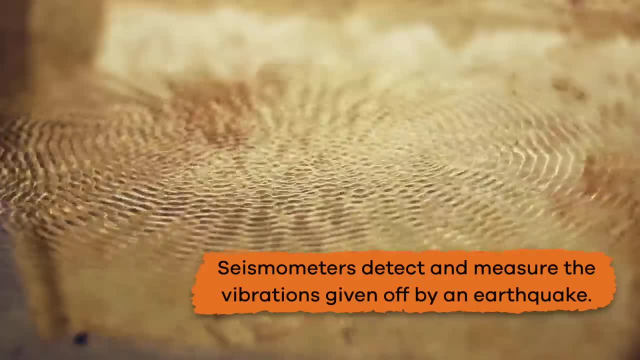 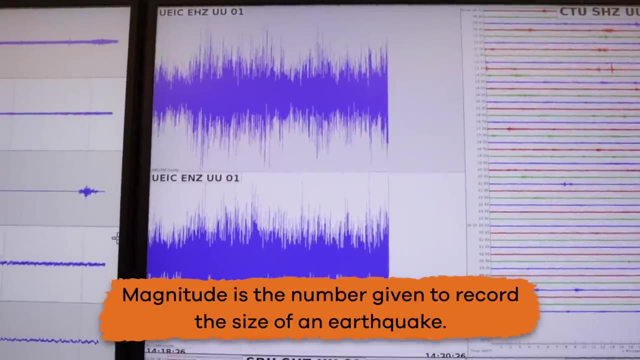 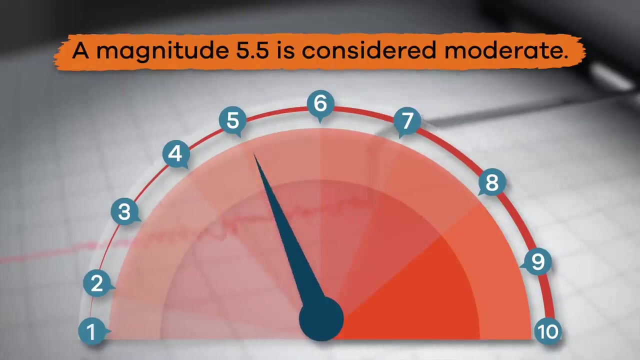 a special device called a seismograph. Seisometers detect and measure the vibrations given off by an earthquake. Magnitude is the number given to record the size of an earthquake. For example, a magnitude 5.5 is considered moderate. Above 8.0 is considered moderate and the magnitude of 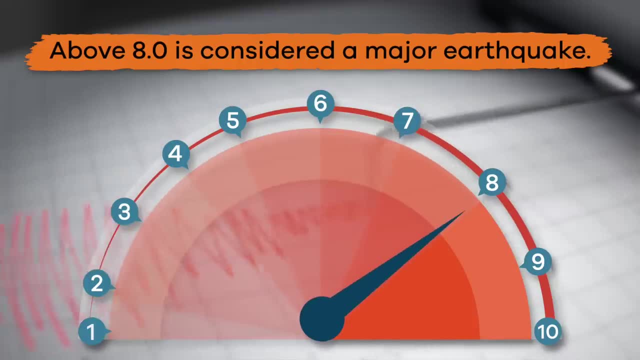 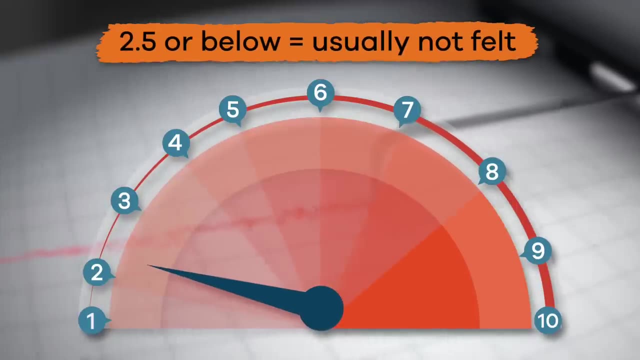 earthquake conditions is considered moderate. It is easy to measure the magnitude of an earthquake: Zero is considered a major earthquake and we see one every year or two. Earthquakes measured at 2.5 or less are usually not felt but can be recorded. 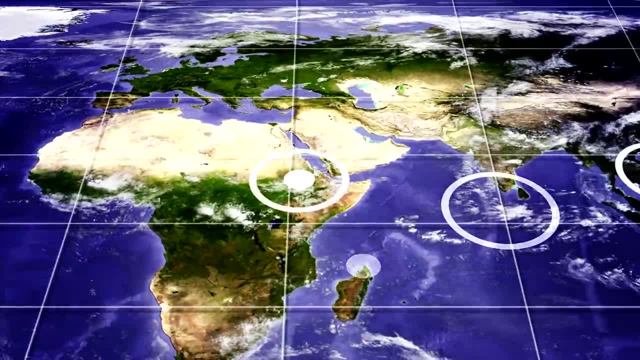 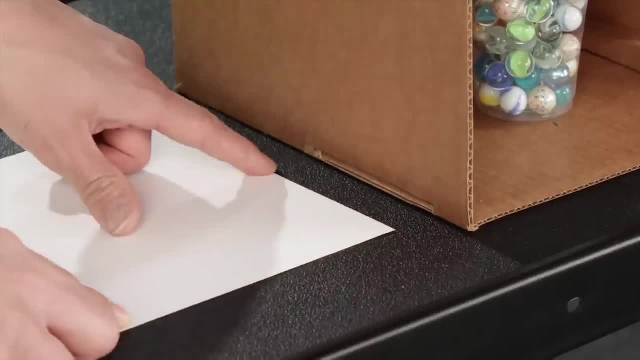 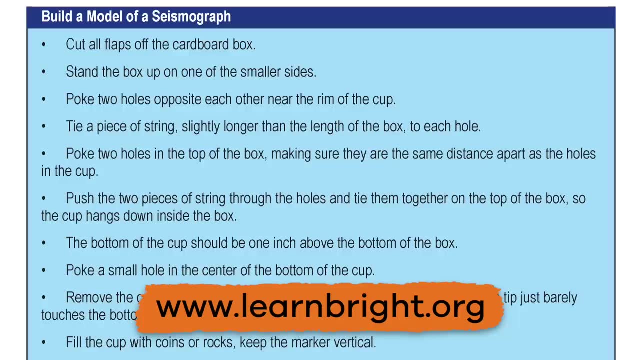 And, believe it or not, there are millions that happen each year. You can make a model of a seismograph at home and we are going to show you how It's activity time. You can print off directions for this one on our website at LearnBrightorg.